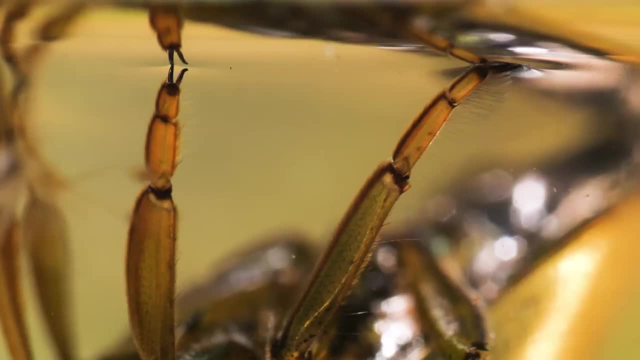 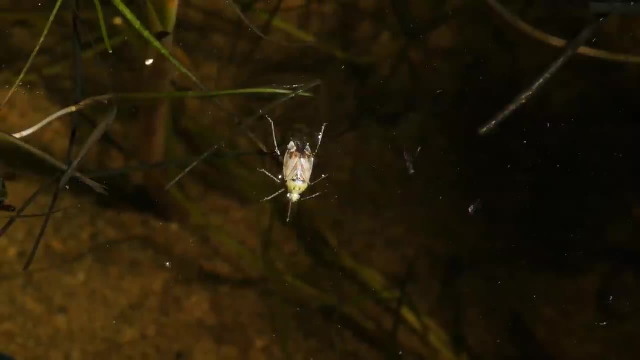 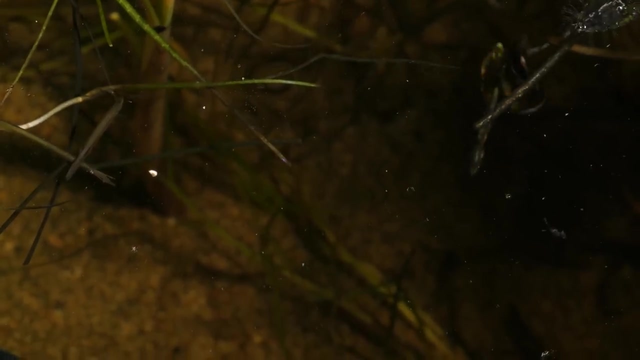 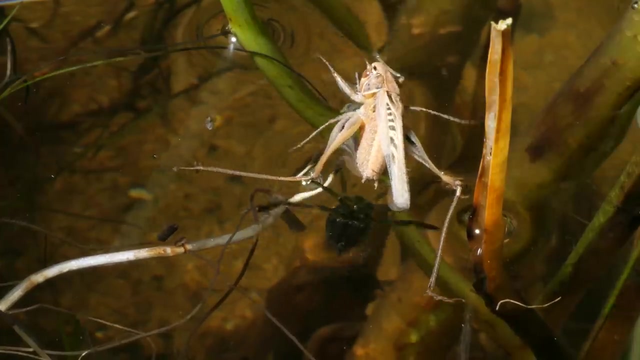 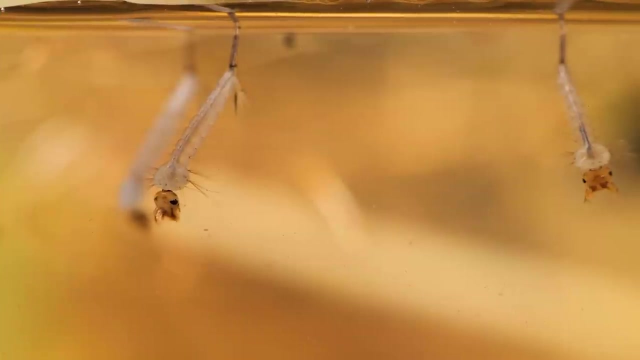 Kinda like they're hanging out on the ceiling. These relentless hunters patrol the shallows in search of unlucky prey and drag them down to a watery death. One of their favorite snacks are these mesquite sticks. Their prey is a mosquito larvae loitering at the surface. 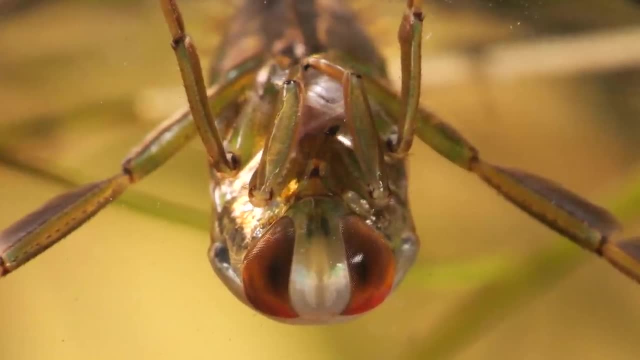 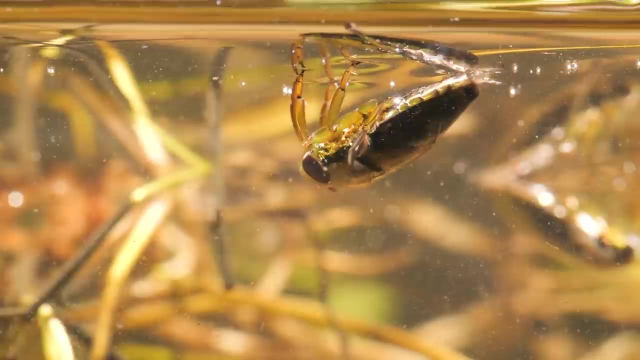 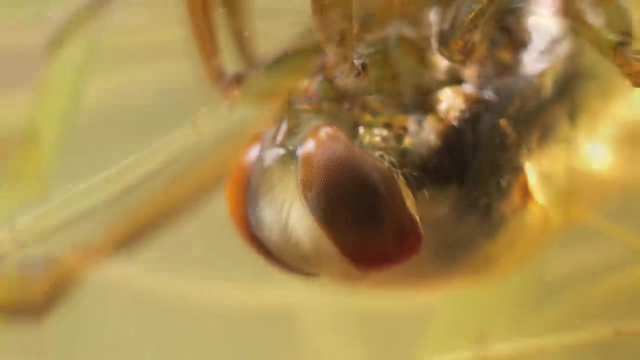 The backswimmer stabs the mosquito with its beak, injecting digestive enzymes and sucking out its meal, leaving an empty husk. But backswimmers aren't the only predators to look out for in these parts, wrap around from the top of their head to the bottom, so they can watch for. 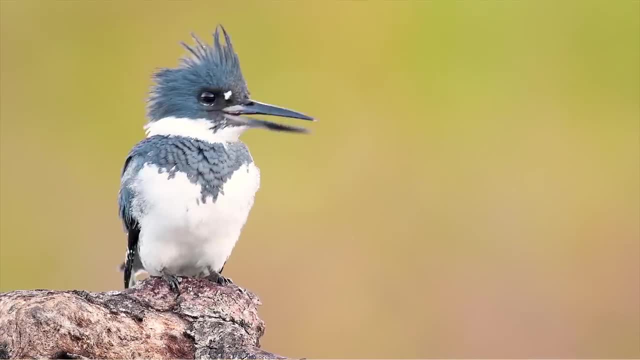 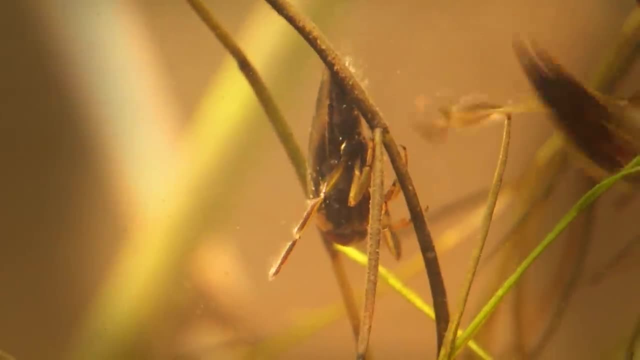 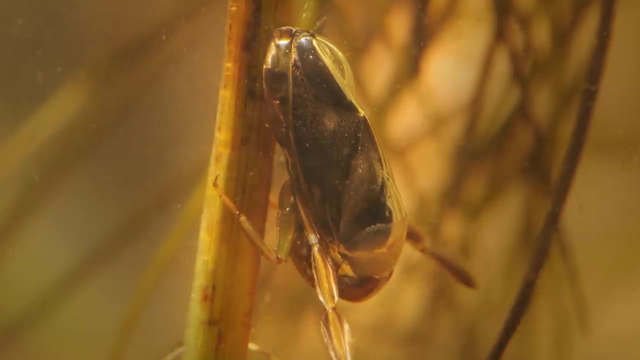 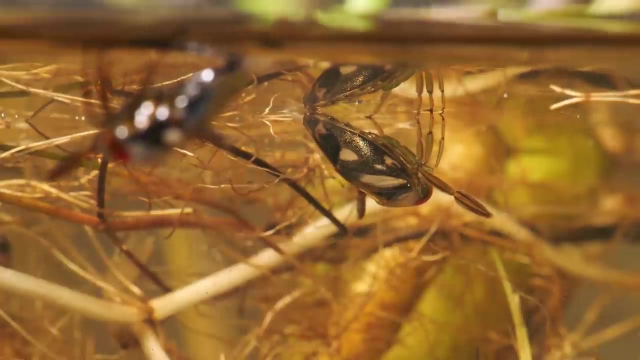 danger below, while keeping their eye on the sky. A single shadow will send them diving for safety in the vegetation, And these bugs can hide down there for a while. They trap a bubble of air around their abdomen that they use to breathe, So they have to hold on to something or they'll pop right back up to the top. 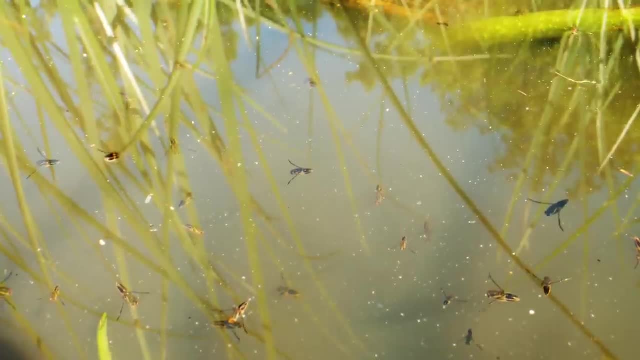 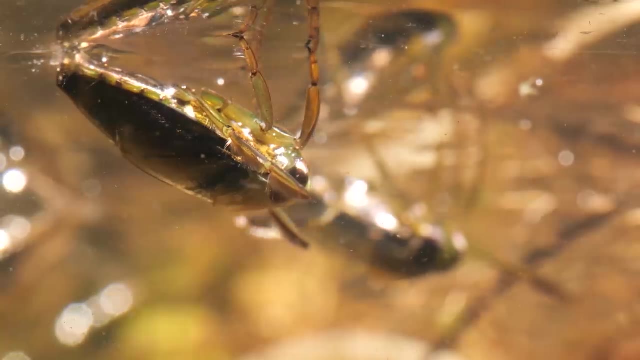 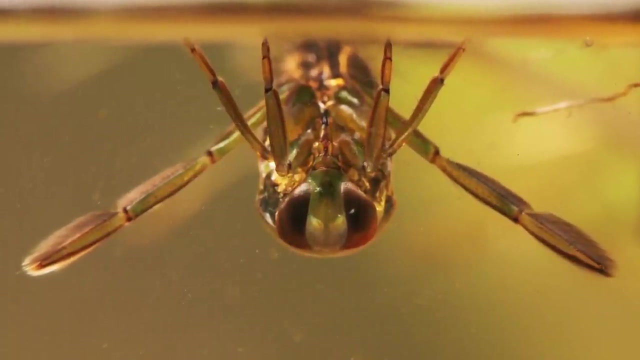 These back swimmers have been hanging out feasting on nearly everyone in sight, But what happens when they start running out of food? They're trapped in this pond, right? Nah, not these bugs. First, they do a very athletic flip, bursting out of the 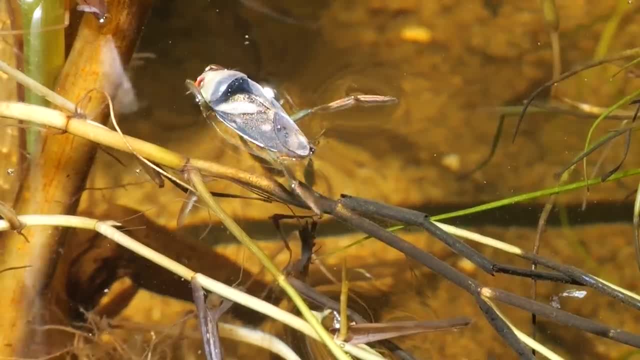 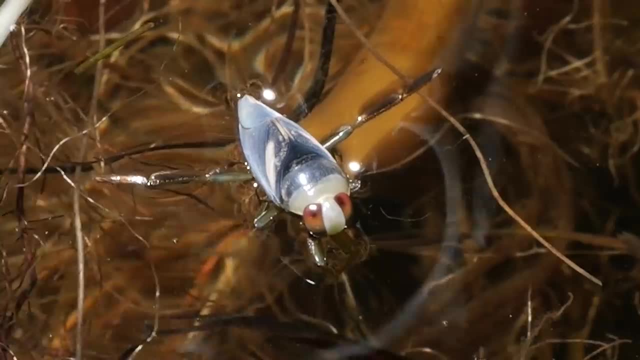 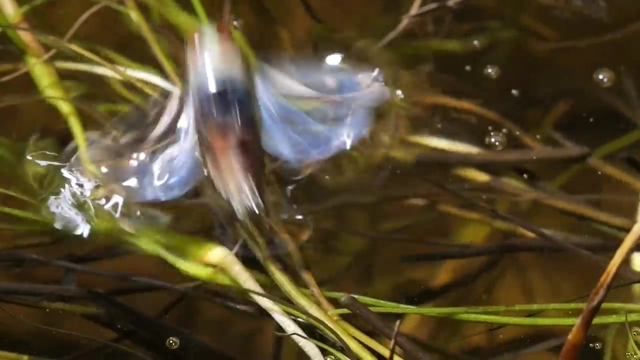 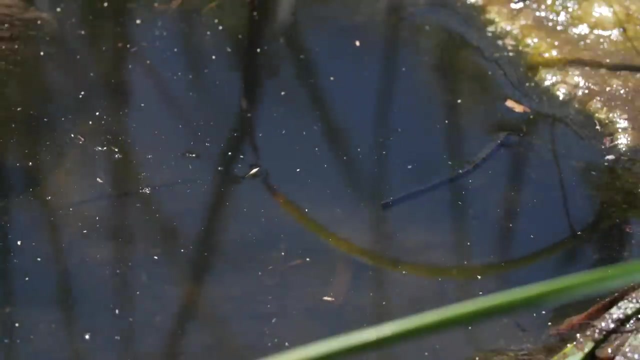 water and, landing on top, They unfurl their wings that they've been hiding, And then they're trapped out of the water for a while, Hiding this whole time under a leathery cover, And take flight, Sometimes traveling for days, in search of a new home. 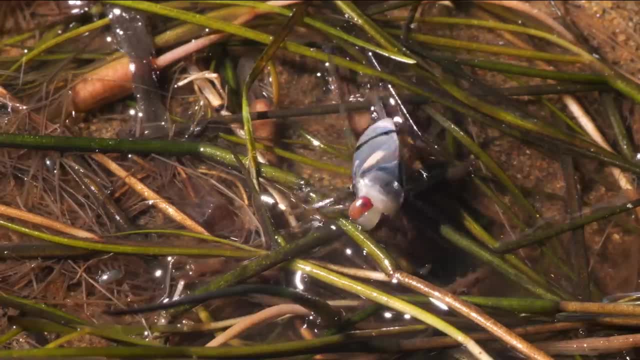 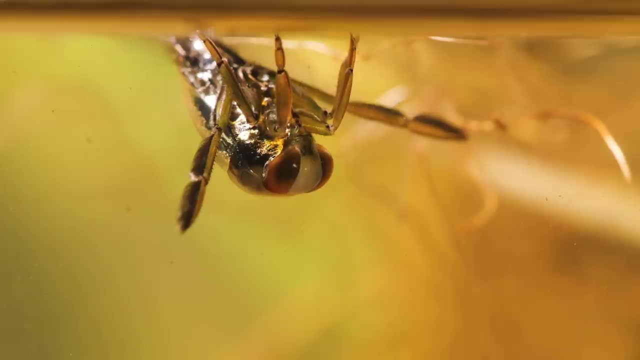 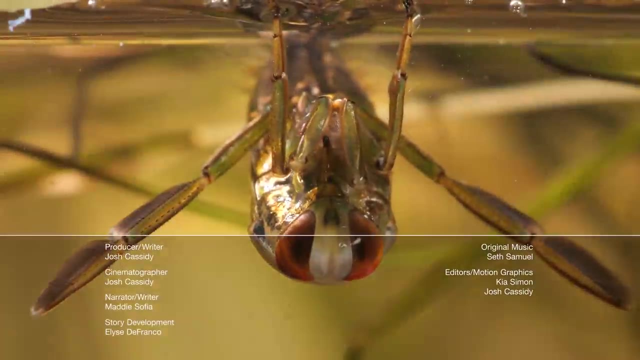 These bugs are often one of the very first creatures to settle in streams, ponds and even swimming pools, Explorers that straddle the boundary between water and sky. Hey, it's Maddie For more freshwater mayhem. check out our Panic at the Pond playlist.